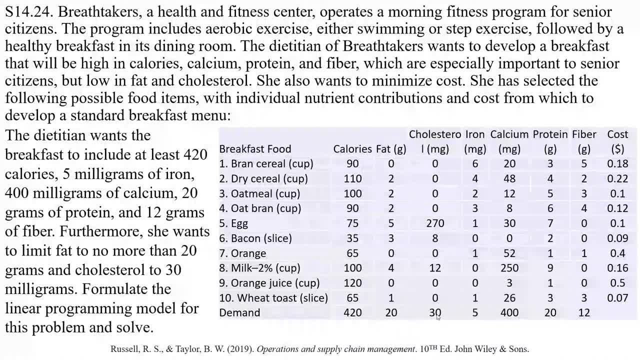 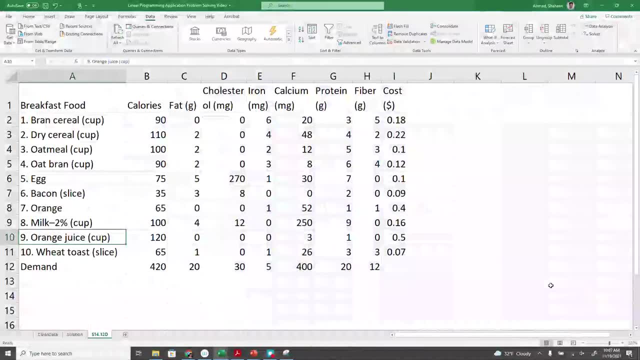 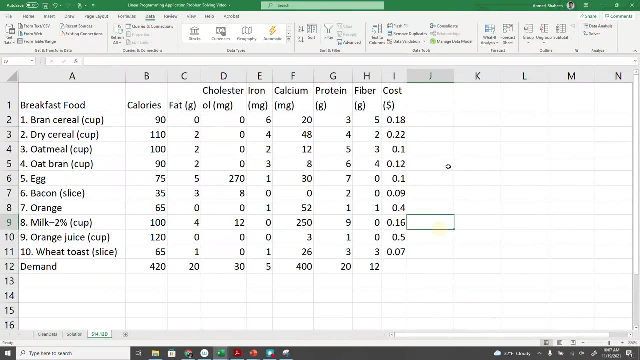 420, and then this fat cholesterol should be less than 20 and 30 and so on. So I'm going to. this problem is taken from the Russell and Taylor 10 tradition, problem number 24.. So I'm going to. we're going to use the Microsoft Excel solver function in solving this. So I have copied the data already. So to start with, we'll have to set the problem in a way or clean the data in a way so we can use. 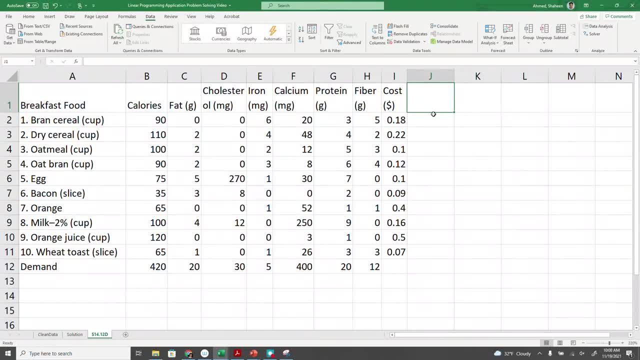 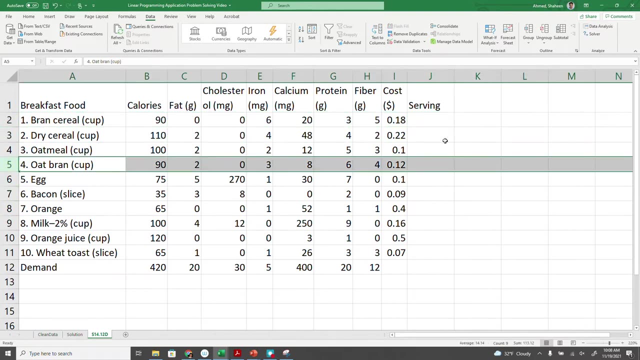 that solver function in Microsoft Excel. So let's say that we're going to see the number of serving for each of these items. We're going to determine that, that how much we'll have to serve to minimize the cost. So, as usual, Excel, start with zeros and then fill these with the optimum number And then the total. 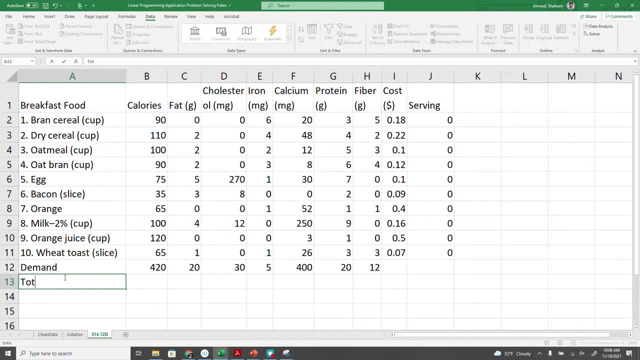 So basically we can use, so a sum product function. basically, if it is a brand cereal, which is 90 calorie per serving, So let's say it uses one brand cereal- This number is replaced by one after this formulation calculation. So then it is going to multiply this. 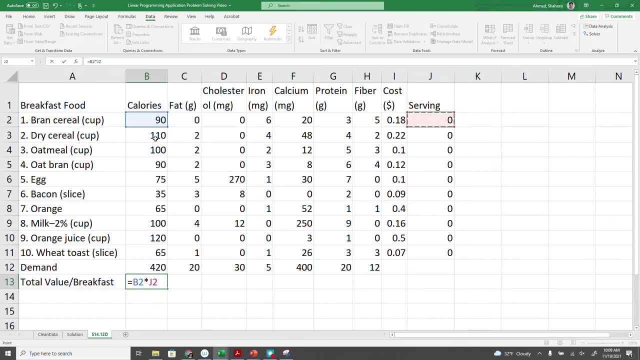 times this plus this times this, and it will keep going like this. Now, instead of that, we can simply do some product. there is a function here that will do that- all this manual operation- for us automatically. So all of these will be marked Oops, So this comma And all of these will be multiplied by this serving. 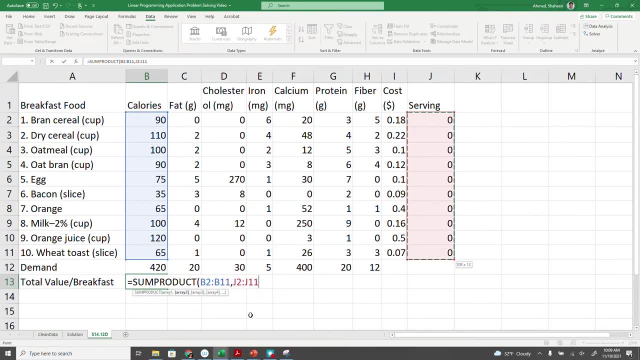 size and then give us the total. So that will be our total calorie. I'm going to use them for fat, cholesterol, iron and everything. So I'll freeze this cell so that I can copy to the next pressing dollar sign before and after, And then we can copy these all the way to the den up to the fiber level. Now the total, also a thing we can copy.